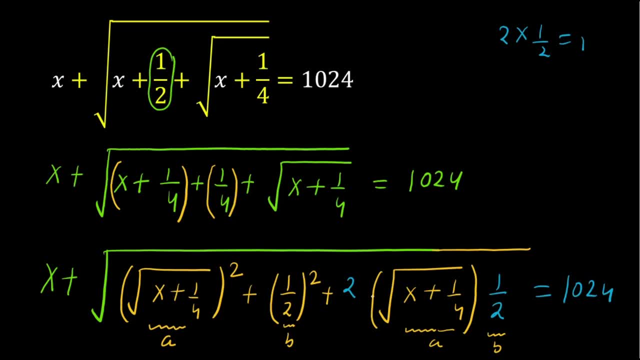 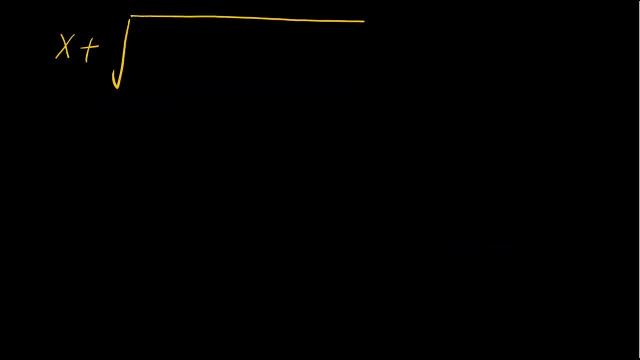 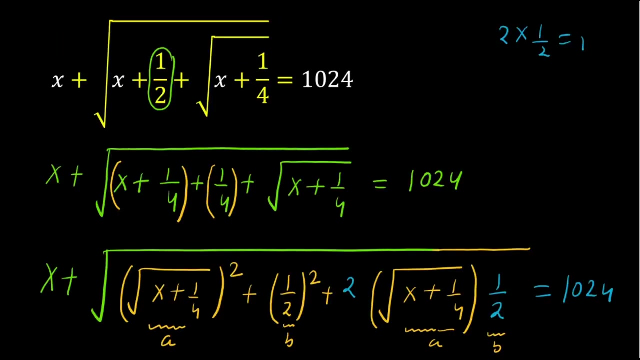 plus 2 times a, b, This is a plus b whole square. So that's why in left hand side, x plus square root of here, value of a is square root of x plus 1 over 4, square root of x plus 1 over 4 plus, and value of b is 1 over 2 here, 1 over 2 whole square, and this is equals to. 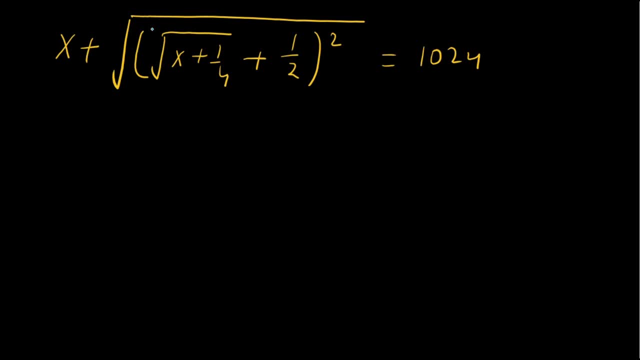 1024.. Now this square root is cancelled out by this square. Then here x plus square root of x plus 1 over 4 plus 1 over 2, and this is equals to 1024.. Now x plus this 1 over. 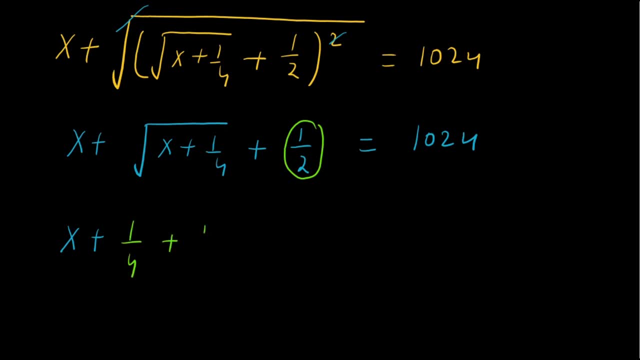 2 is same as 1 over 4 plus 1 over 4.. Now, x plus this, 1 over 2 is same as 1 over 4 plus 1 over 4, and this is equals to 1024.. Again, x plus 1 over 4 is same as square root of x plus 1 over 4. bracket power: 2 plus this. 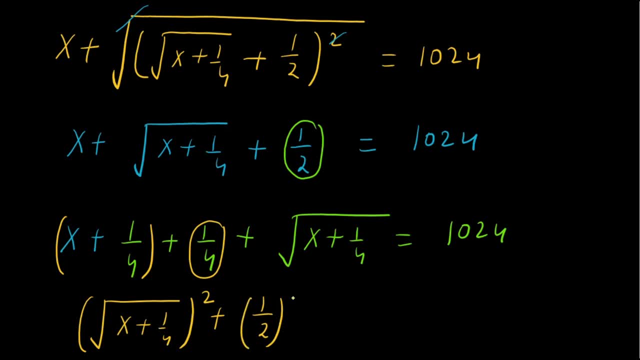 1 over 4 is same as 1 over 2. bracket power: 2 plus square root of x, plus 1 over 4 plus 1 over 4.. Here, if we multiplied by 2 and multiplied by 1 over 2, and we know that 2 times, 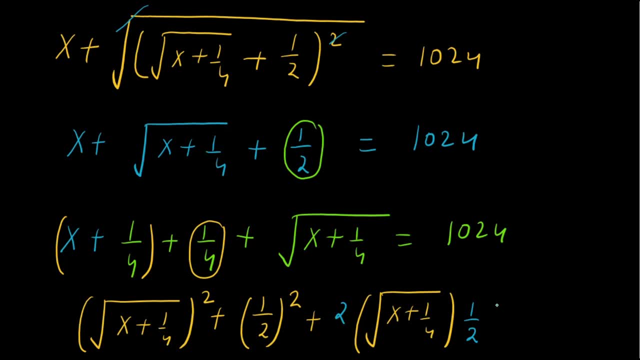 1 over 2 is 1 and 1 is multiplied by any number, then number is not changed and this is equals to 1024.. Again, if you assume square root of x plus 1 over 4 is a and this 1 over 2 is b. 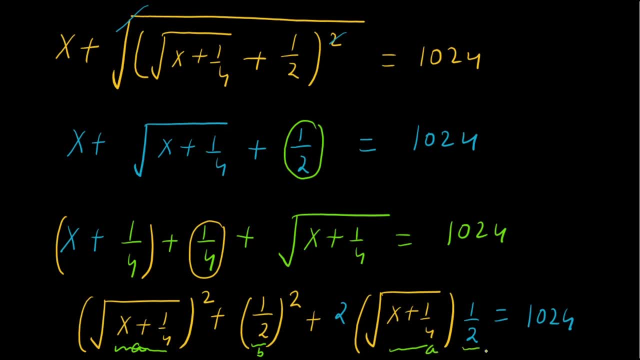 and this expression is a and this 1 over 2 is b. So this is equal to 1024.. So this is equal to 4.. 2 times 1 over 2 is b. then a square plus b, square plus 2 times ab, and we know that.